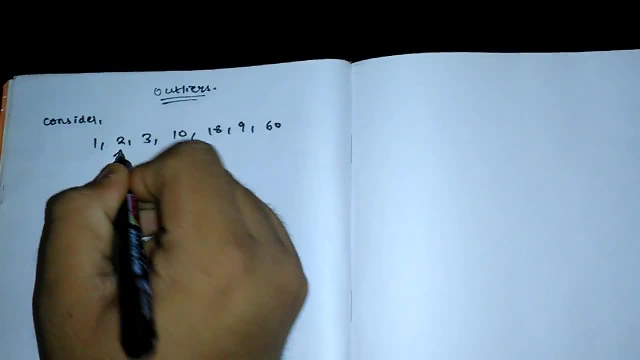 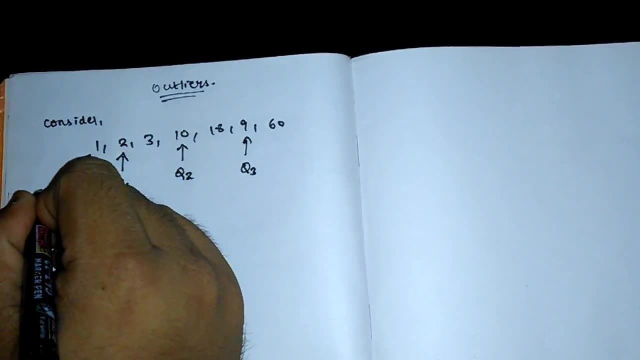 which divides the given sequence into 2, equal half. 2 is the lower quartile value, which is denoted by q1, 9 is the upper quartile value, which is denoted by q3, 1 is the lower extreme value and 60 is the upper extreme value. this is how we plot. 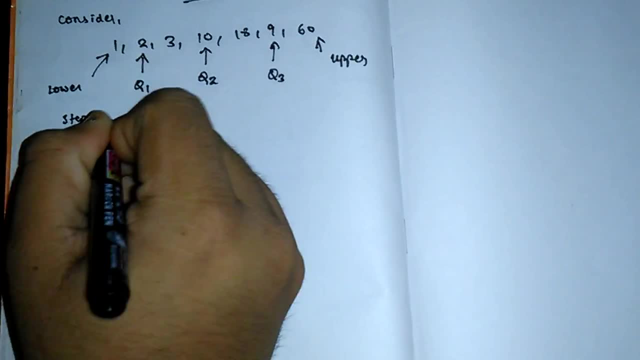 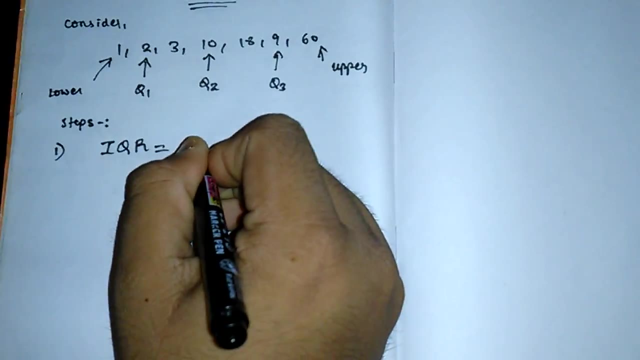 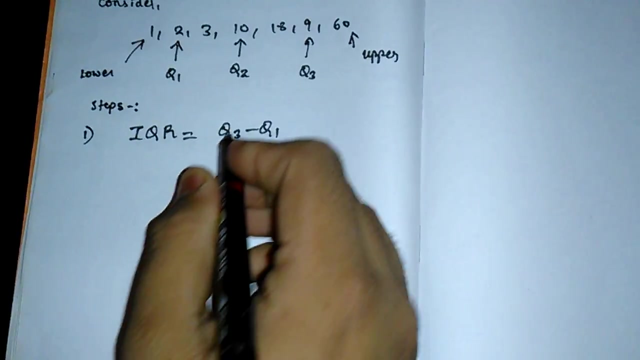 a box plot. now the steps required to detect an outlier are given by. first of all, we have to calculate the interquartile range. IQR is given by q3 minus q1, which is the subtraction of the upper quartile value minus the lower quartile value in this given sequence. 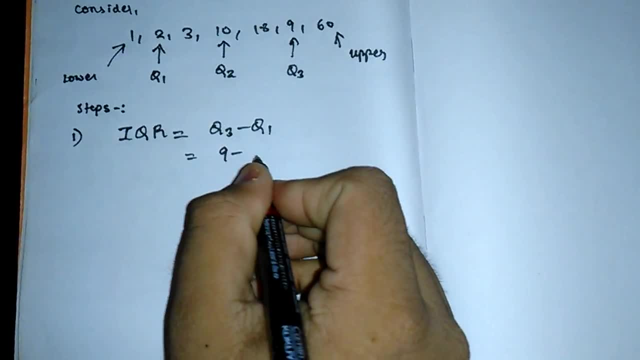 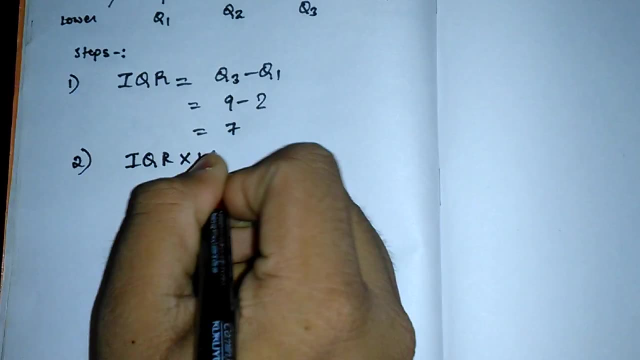 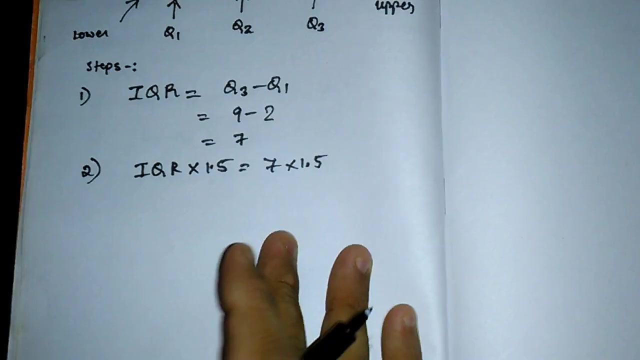 the upper quartile value is 9, minus the lower quartile value, which is 2, which comes out to be 7. now we have to multiply the interquartile range into 1.5, which comes out to be 7, into 1.5, which comes out to be 10.5. now the third step. 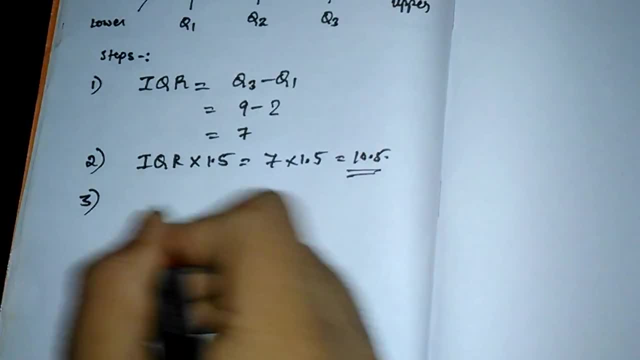 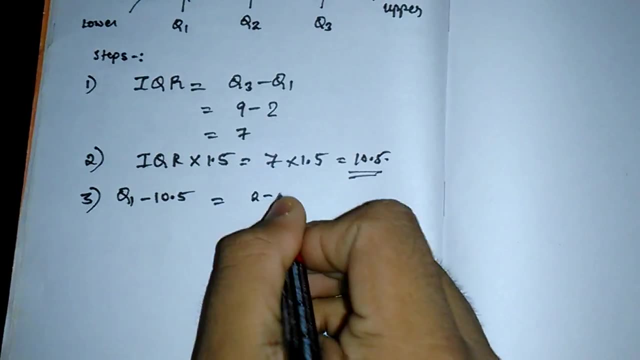 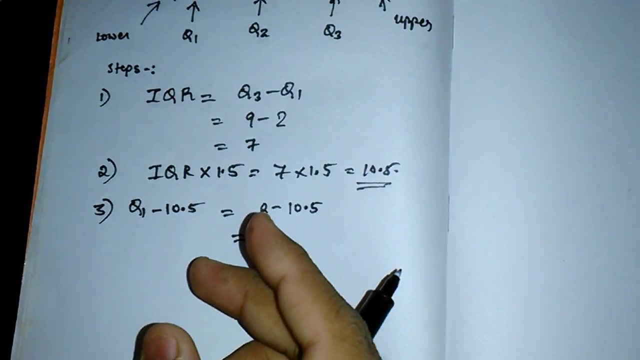 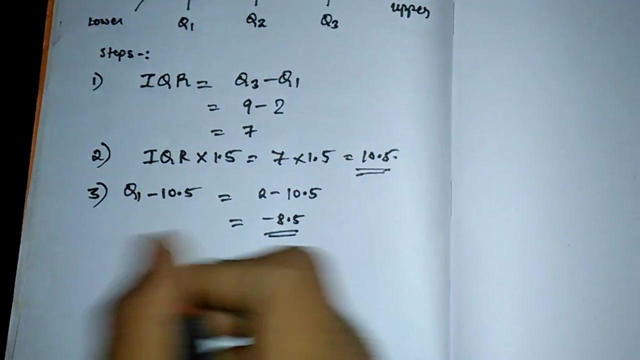 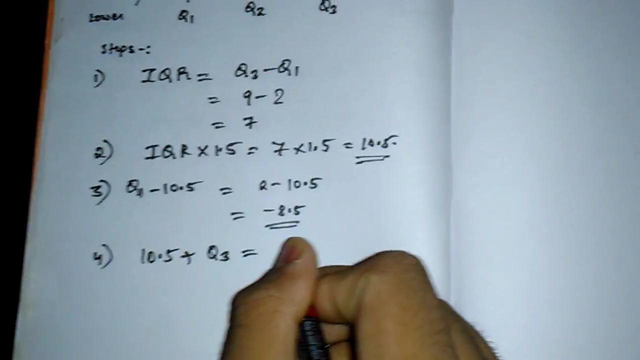 is to subtract the 10.5 value minus the lower value, which comes out to be 2 minus 10.5, which comes out to be minus 8.5. the fourth step is to add the 10.5 value to the upper quartile value, which comes out. 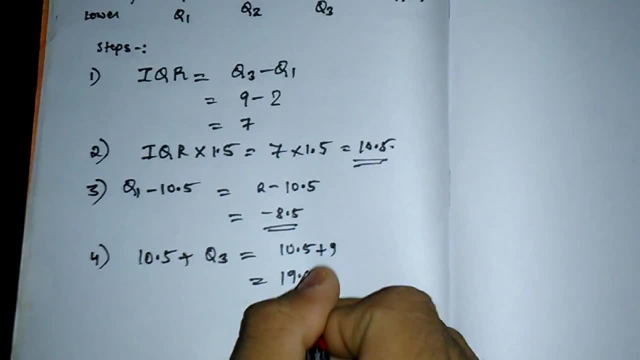 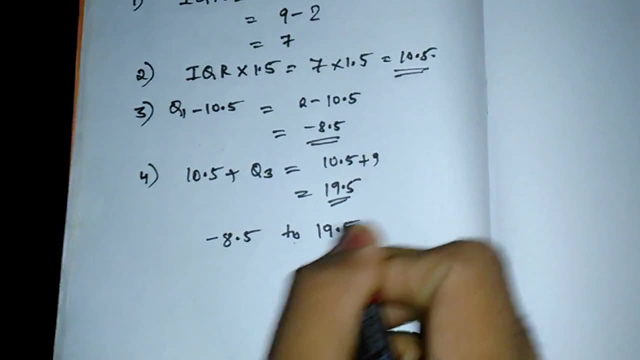 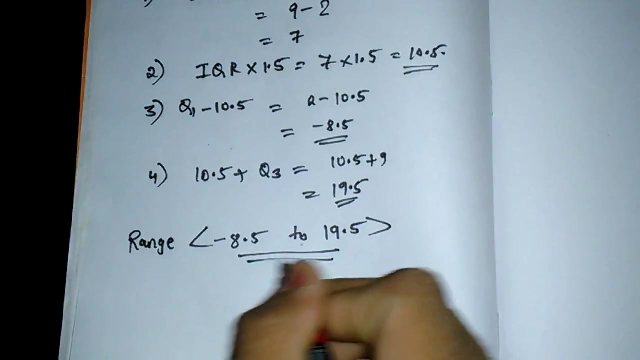 to be 10.5 plus 9, which is 19.5. now the two values which we got is 8.5 to 19.5. now this is the given range which is required to detect whether the given number is an outlier or not. if the number lies below minus 8.5 and is: 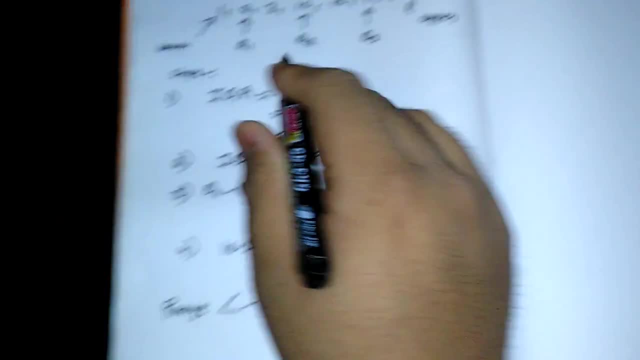 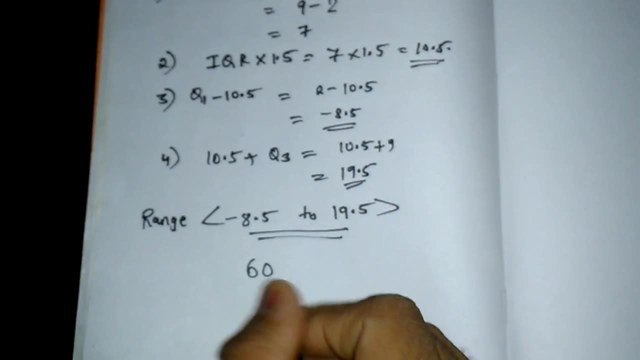 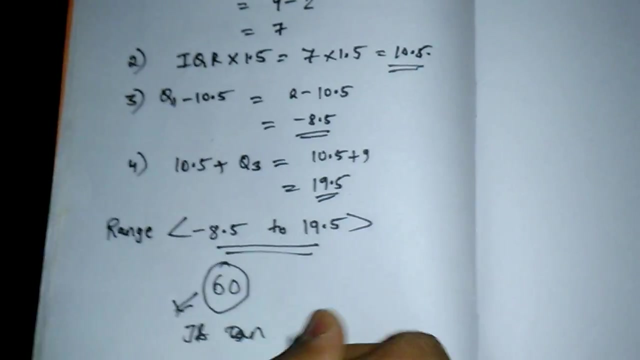 greater than 19.5, then it is an outlier from our given sequence. 1, 2, 3, 10, 18 and 9 all satisfy this range, but 60 is greater than 19.5. therefore, in this case, 60 is an outlier if the value: